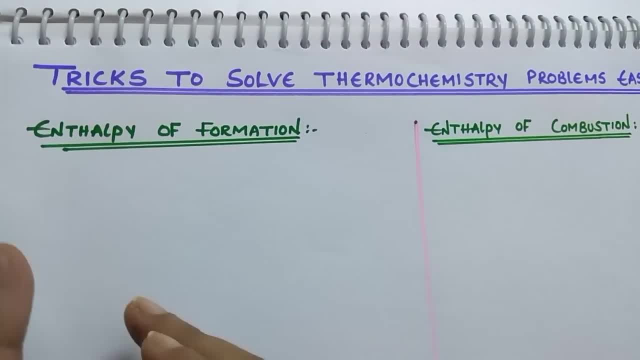 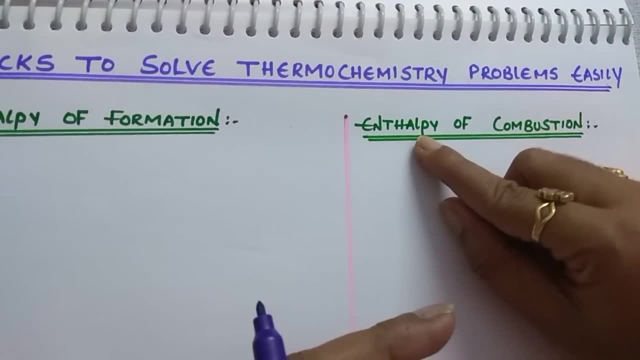 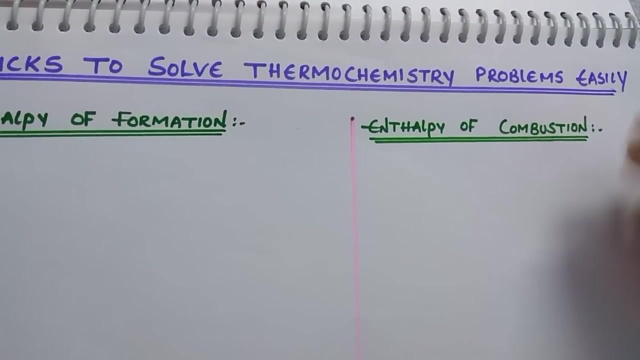 during the formation of one mole of a compound from its constant elements. We call it as enthalpy of formation. What is enthalpy of combustion? It is the enthalpy change during the combustion of one mole of a substance. We call it as enthalpy of combustion. This we generally do in the presence. 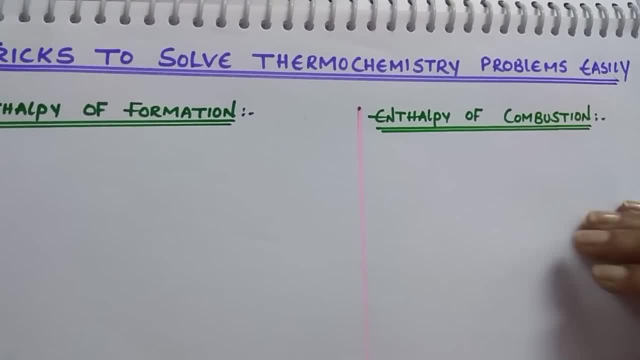 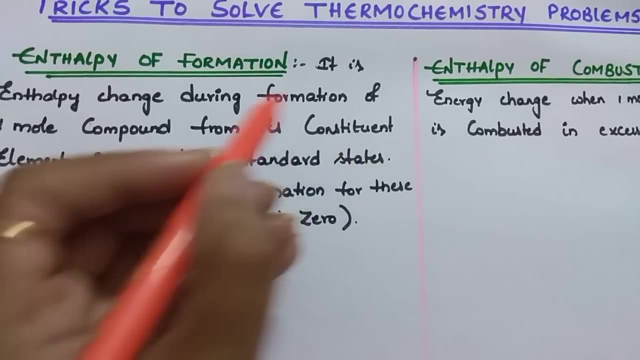 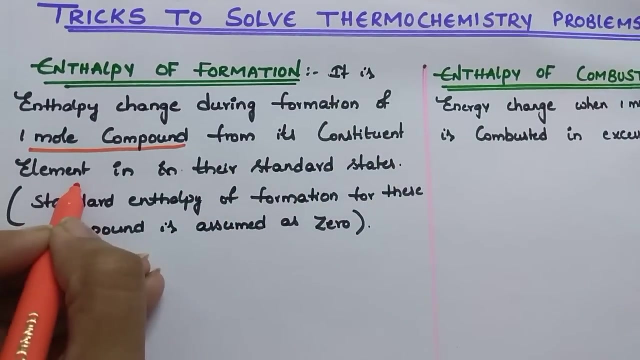 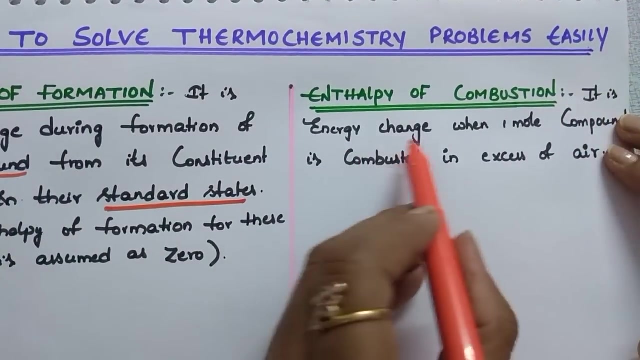 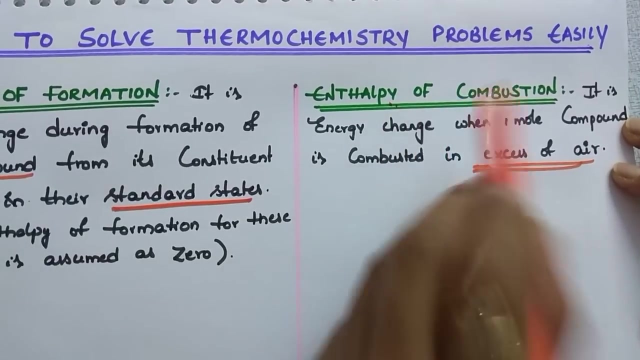 of excess amount of oxygen. Let us see the definitions. It is enthalpy change during the formation of what Students one mole of compound from its constituent elements which are, in their standard states, Clear, And here it is energy change when one mole of a compound is combusted in excess of air. That is called enthalpy of combustion. 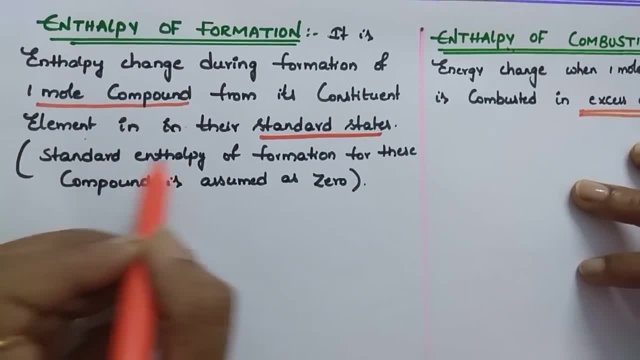 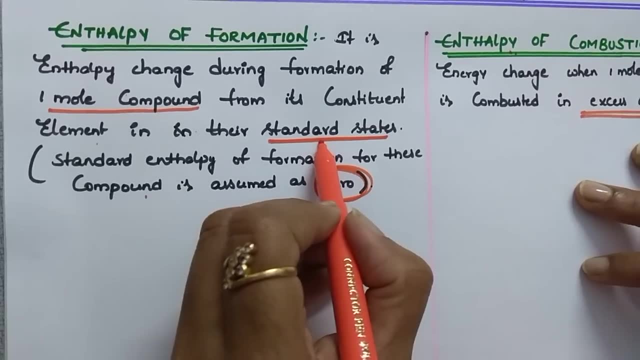 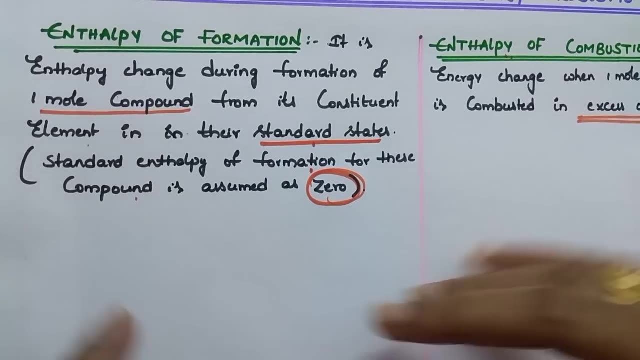 Here I used standard states, and standard enthalpy of formation for these compounds is assumed as zero. Which one for standard states? What are these standard states? Standard states is nothing but the presence of element in their purest form in the nature. We call it as standard states. 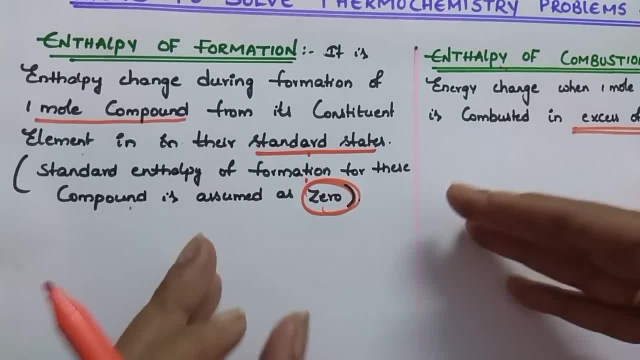 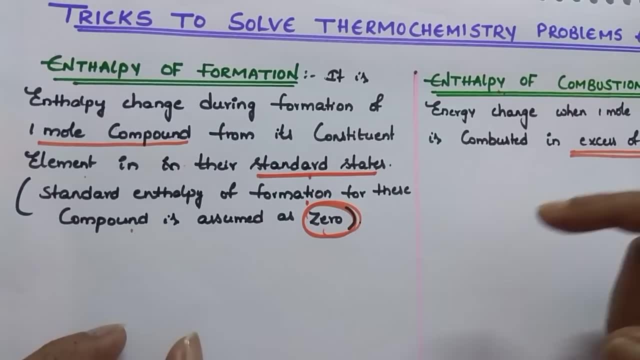 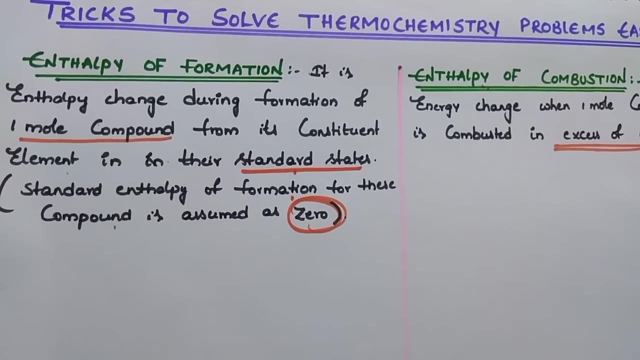 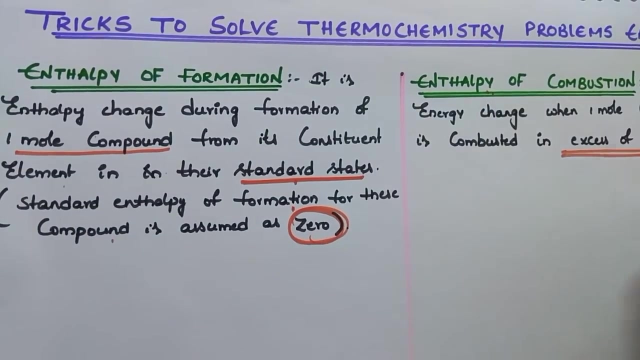 For example, carbon present as a graphite. This is the most standard state when compared to diamond, because carbon in the graphite state is thermodynamically more stable than the diamond. That is the reason only graphite is considered as a standard state Carbon. I am going to give you few list. See here. this is most important. 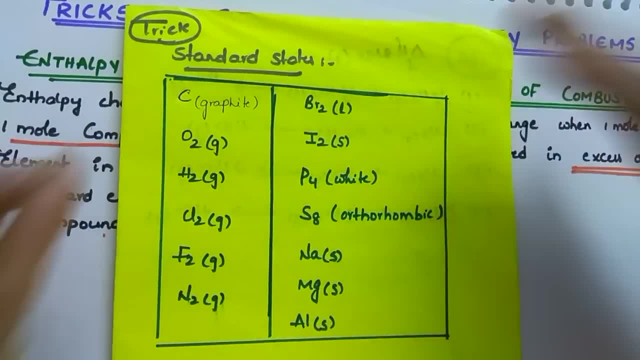 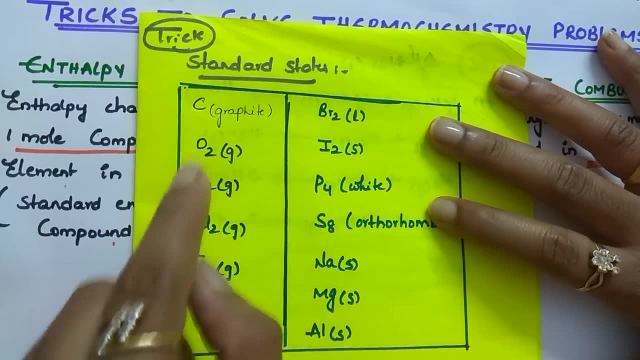 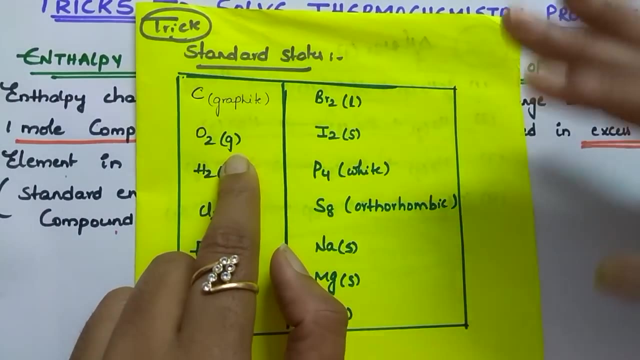 This is very, very important. Note this list and keep with you while solving this thermochemistry problems. It will help you. Carbon exists as a graphite state and oxygen present in as O2 in the gaseous state in nature. You have to take only this form as a standard state. 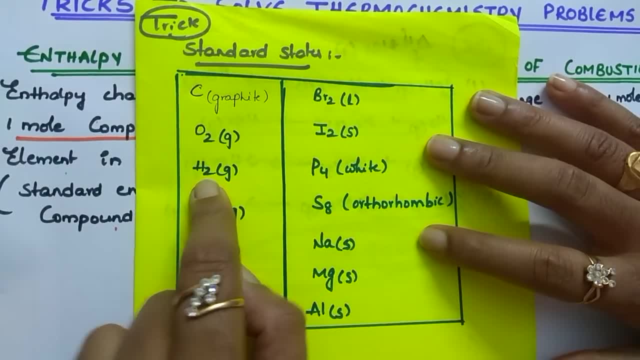 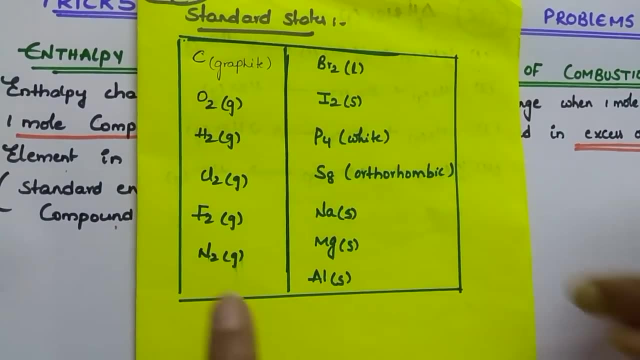 not O3 as a standard state for oxygen Hydrogen present as H2 in gaseous state. Chlorine present as Cl2 in gaseous state. Fluorine present as F2 in gaseous state. Nitrogen present as N2 in gaseous. 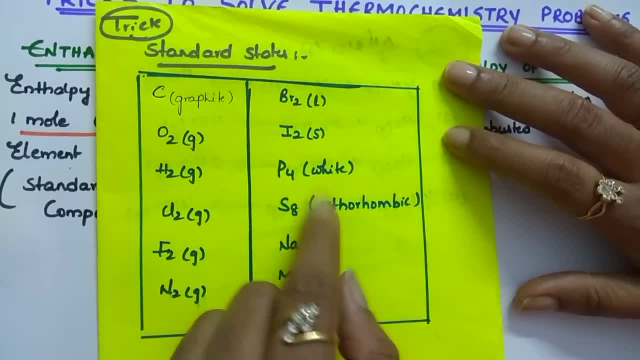 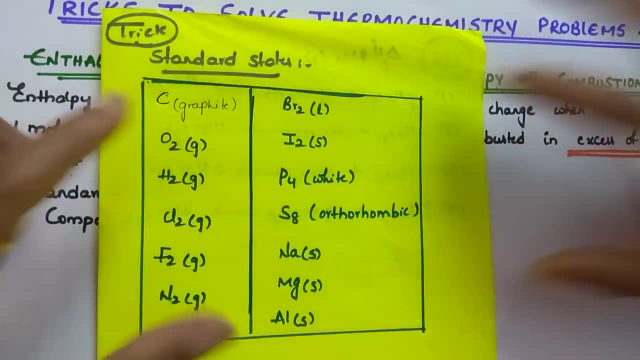 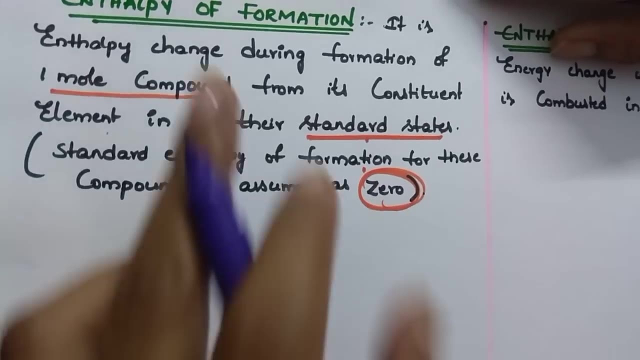 state. Bromine present as a liquid in gaseous state. Sorry, bromine present as Br2 in liquid state. Iodine present as I2 in solid state, Like this. this data is very, very important. And coming to this, how to write the standard? enthalpy of formation? First, what is a standard? 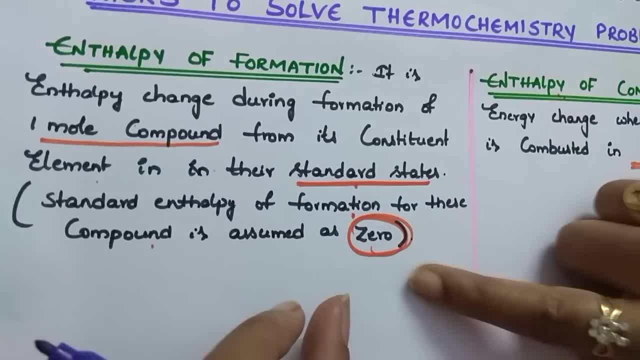 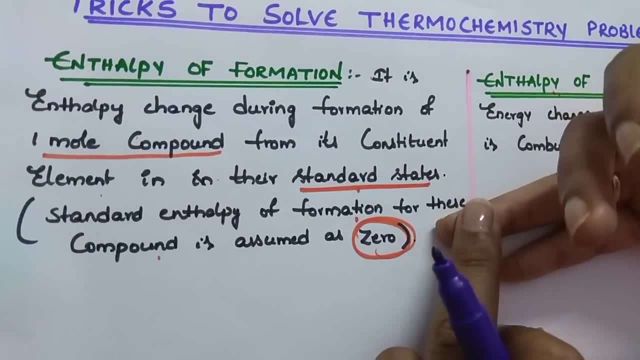 enthalpy of formation. What is the difference between enthalpy of formation and standard Means? whenever the reaction is taking place at standard conditions, like 1 bar pressure and 1 molar concentration and temperature, usually like 25 degree Celsius, we call it. 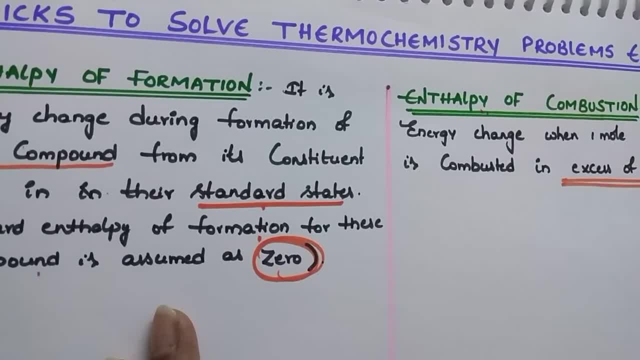 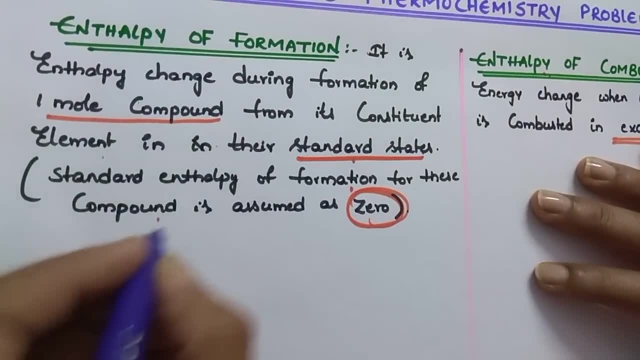 standard enthalpy of formation, In the same way standard enthalpy of combustion also, even in the same conditions. we call it as standard enthalpy of combustion. Let us see this how we represent this: enthalpy of formation is delta, because change in enthalpy we are. 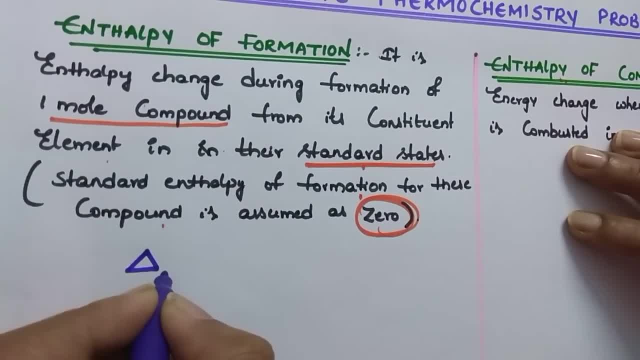 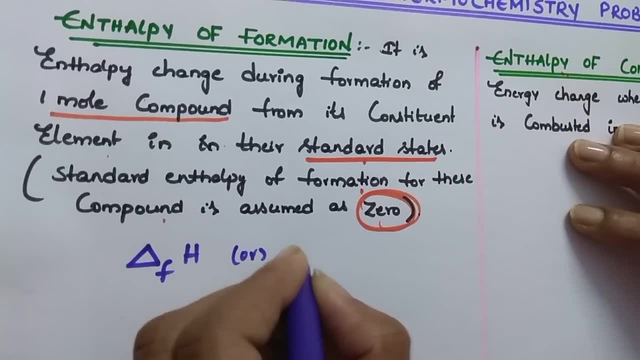 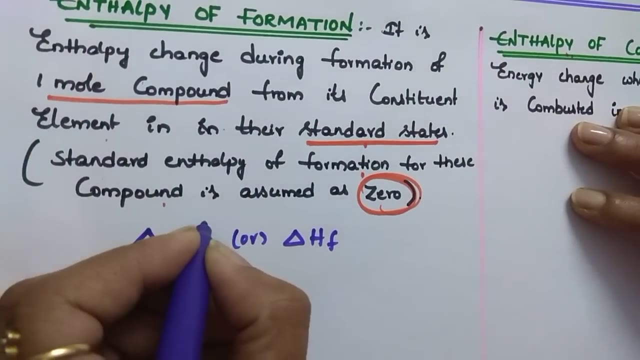 going to find, because we cannot find the absolute enthalpy, delta F of H, What it means We can write in this way: also delta HF. This is the representation of enthalpy of formation For standard enthalpy of formation. 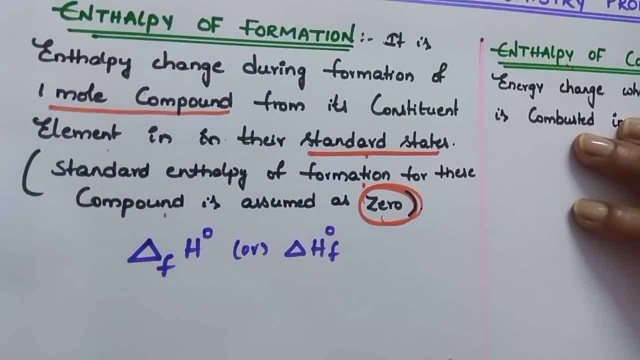 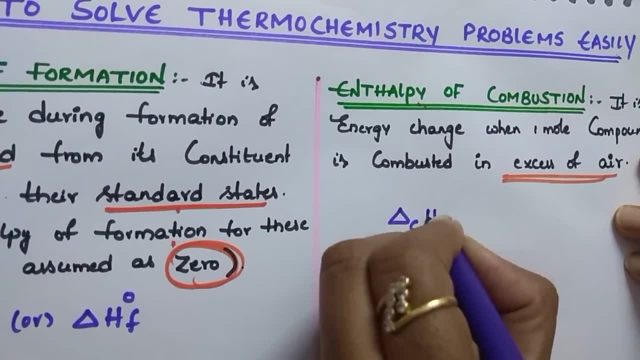 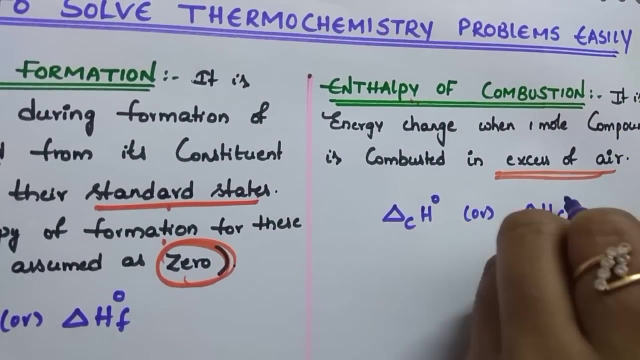 just to put note here, then, which stands for standard enthalpy of formation. In the same way, enthalpy of combustion is delta CH or delta HC. How to write standard enthalpy of combustion is just put note here. This is called, as this is the representation of enthalpy of formation, and 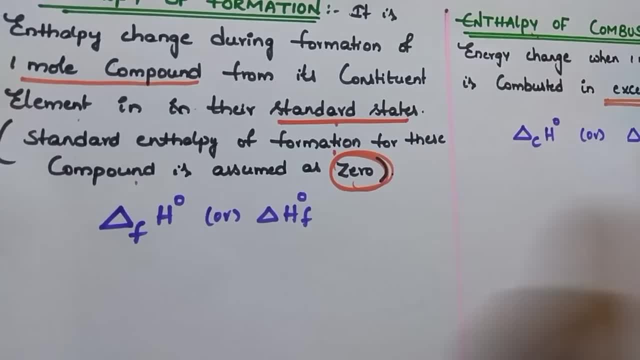 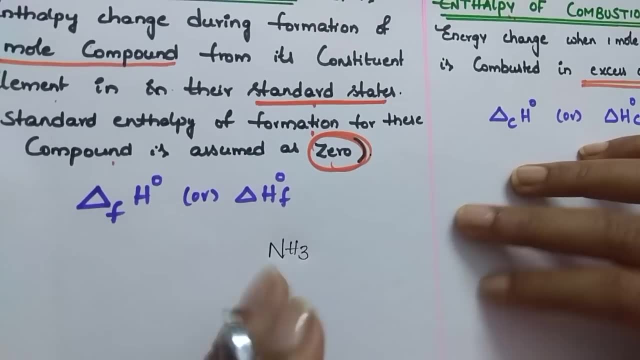 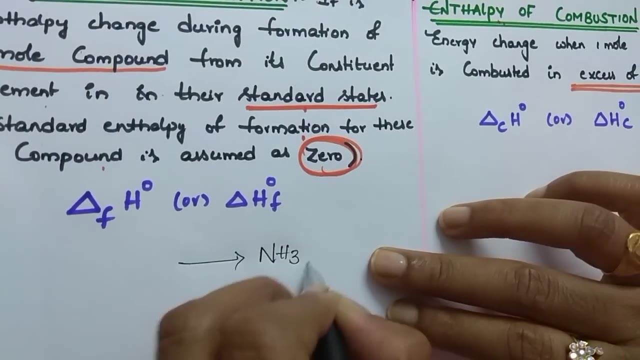 enthalpy of combustion. Here I am going to discuss the most important point. See here, students, if you want to do the formation of 1 mole of ammonia, write this: 1 mole of ammonia in the product side Clear. Suppose you want to prepare gaseous ammonia. What are the reactants? what are the elements? 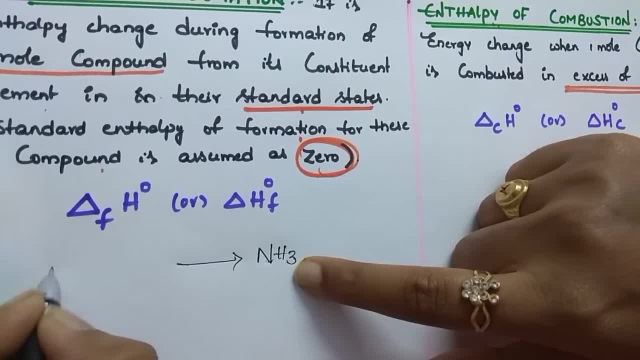 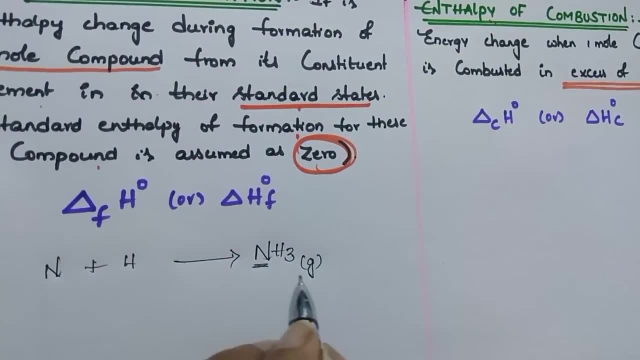 which is having nitrogen and hydrogen. What you have to do is write nitrogen N here and hydrogen H here, Clear. But nitrogen exists, as in which form I told you, in the nature. you have to take that, only nitrogen as N2.. 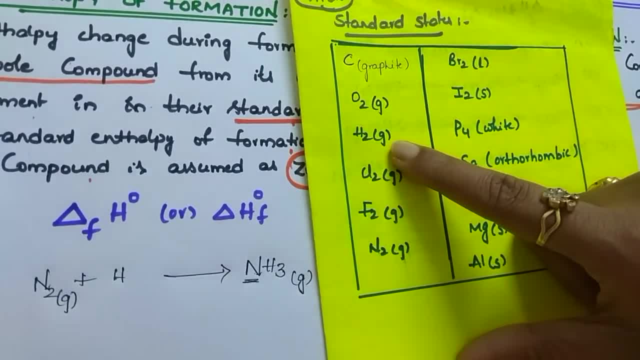 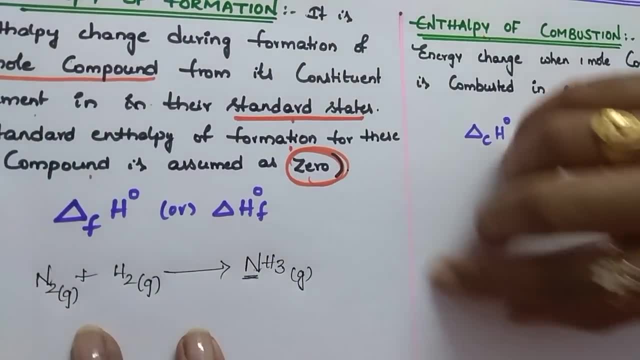 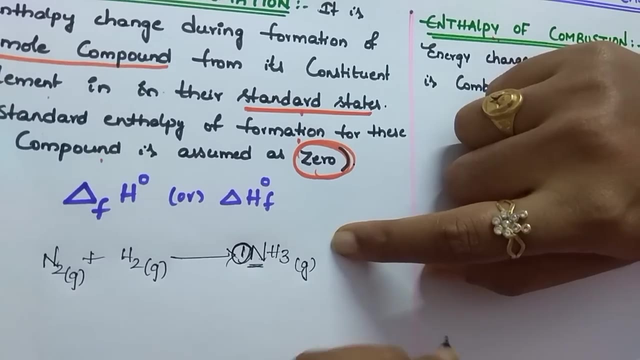 H2 in gaseous state and hydrogen is present as H2 in gaseous state. You have to take that only Clear Now. next important trick while writing this reaction is: we want to do the formation of ammonia, only 1 mole. So here the coefficient is only 1 mole, According. 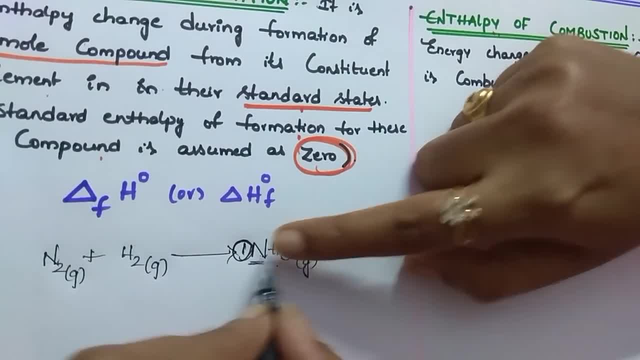 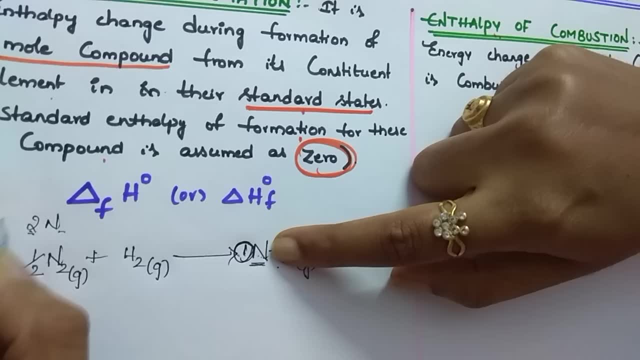 to this. you have to balance the reactants. Got the clarity Nitrogen, only 1 nitrogen, but here is 2, is there? So take half, because how many nitrogen sent to me is 2. 2 nitrogens. 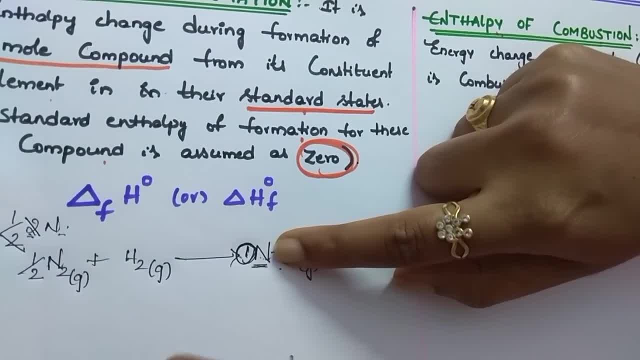 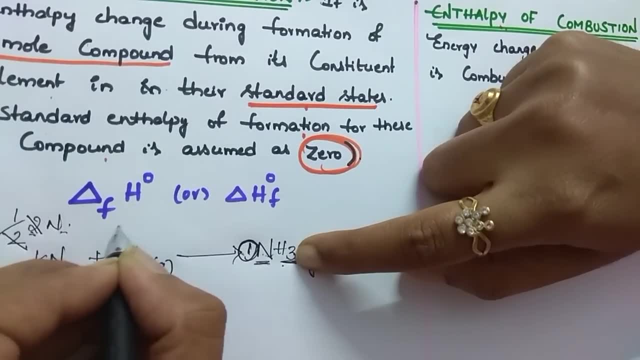 If you take, half gets cancelled, then only 1 nitrogen will be left And in the same way H2, how many are there? 3 here Here, 2 hydrogens only there. So take 3 by 2 means 2 hydrogens. 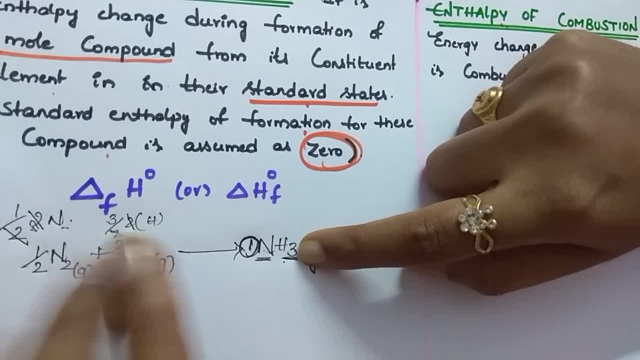 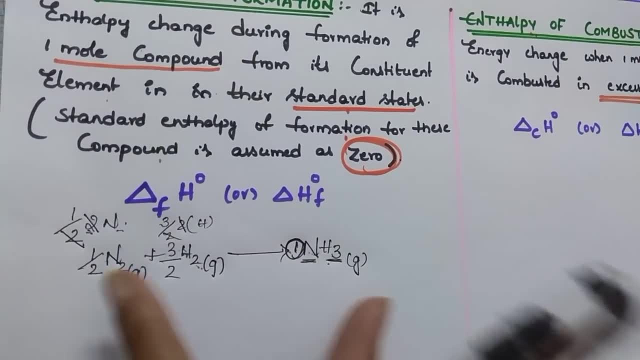 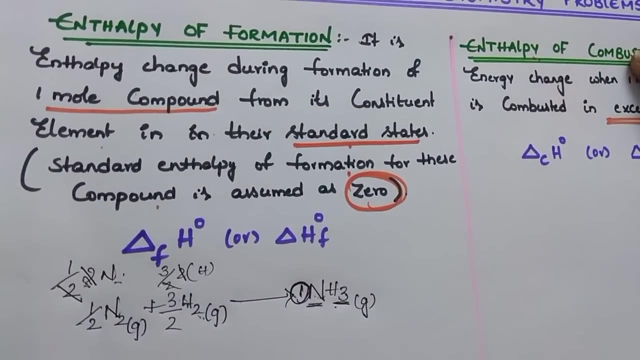 and you are taking 3 by 2 gets cancelled. What will be left? 3 means which means 3 by 2. H2 means 3 hydrogens. This is the exact equation. Enthalpy of formation. reaction of ammonia. This kind of reaction- writing is most important in thermochemistry chapter. 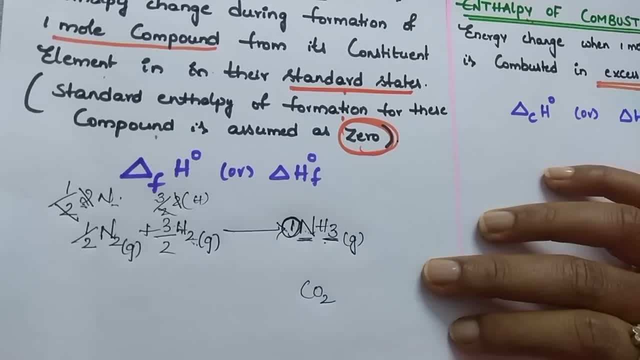 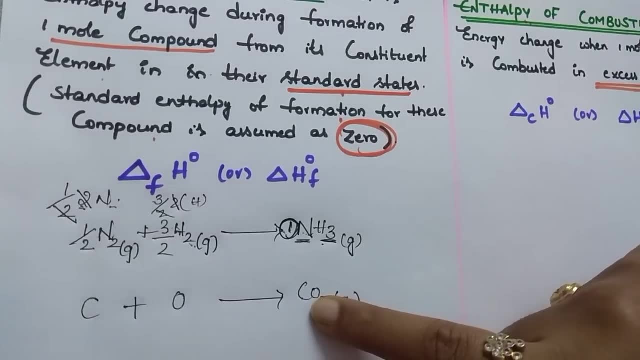 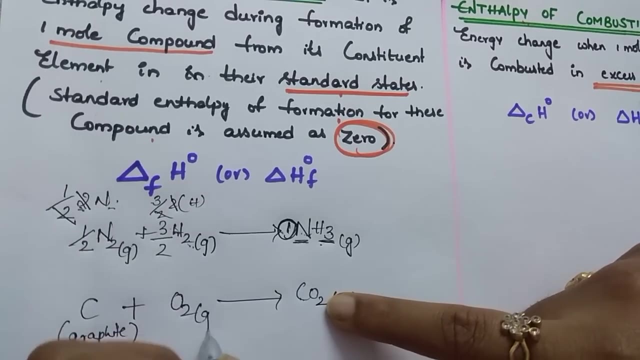 See here, if you want to do the formation of 1 mole of CO2, how to write this reaction. CO2 gas, if you want to prepare, means elements carbon and oxygen. After that, what are the standard states? Carbon graphite is the standard state. Oxygen O2 in gaseous state is the standard. 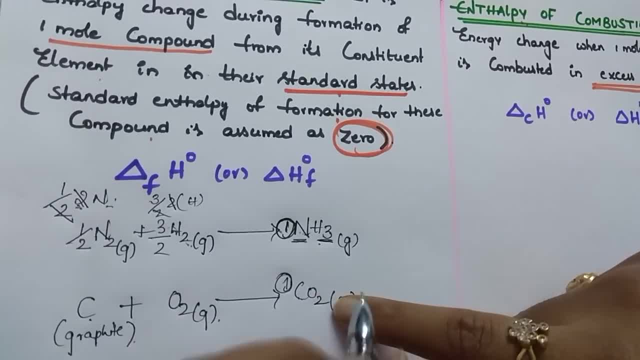 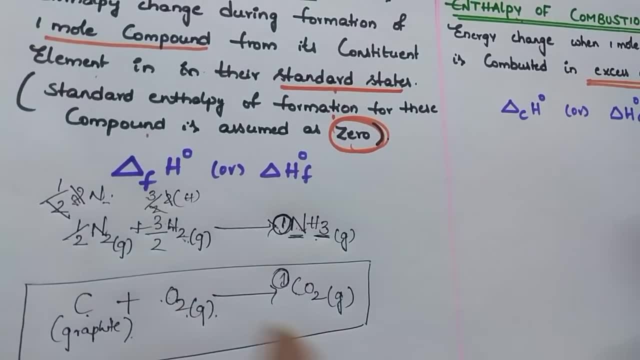 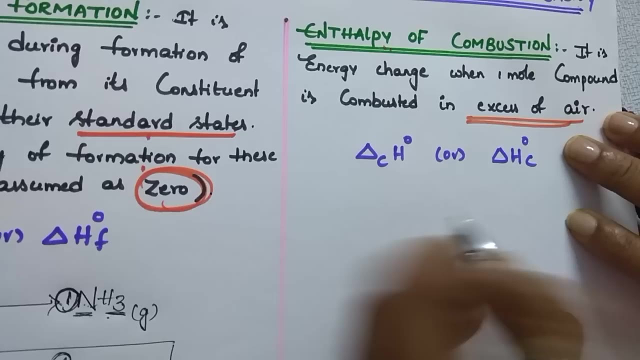 state: This is 1 mole, So carbon is 1 mole. and oxygen? how many are there? 2 is there, So O2.. That's it. This is the standard equation. Learn this, Take different examples and learn writing of formation reactions. Let us see the combustion, For example. you want. 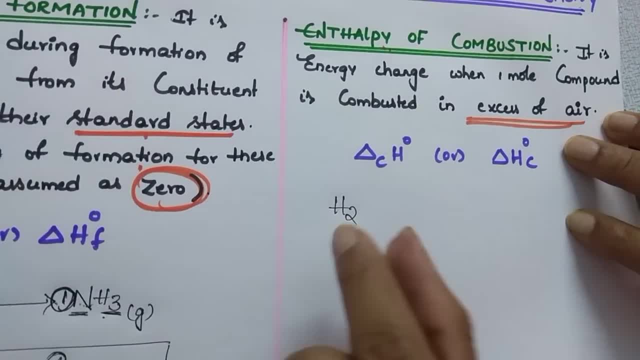 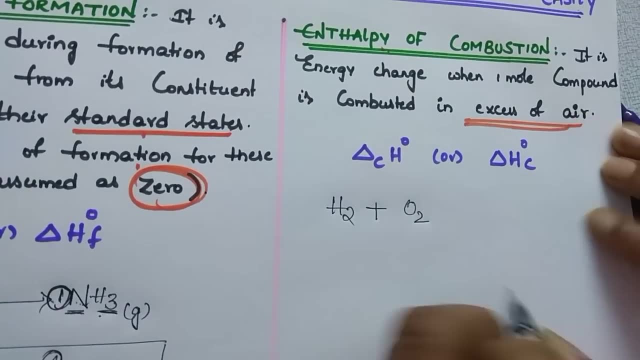 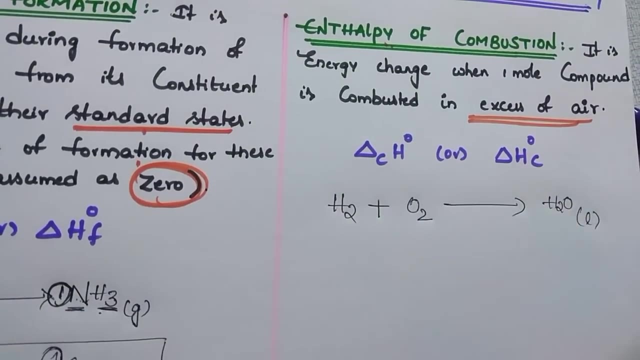 to do the combustion of H2.. Then take what you are going to do, the combustion product side. This reaction takes place in excess of oxygen, So write O2 and in the product side write H2O. I am taking as liquid Why? Because at room temperature H2O exists as. 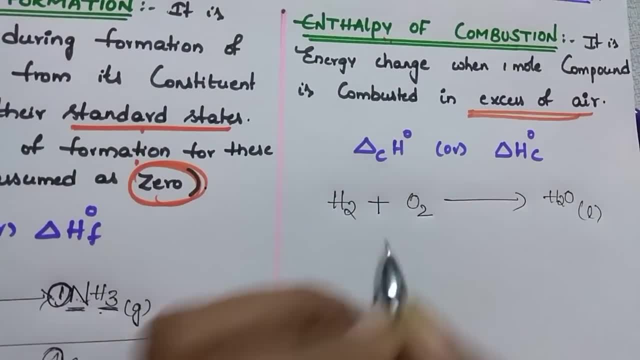 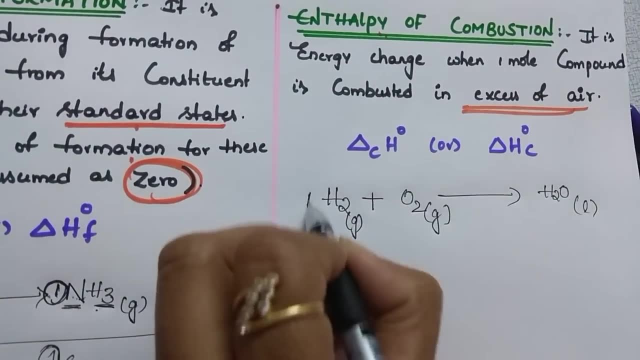 a liquid only. That is the reason I am taking H2O liquid And H2, standard state is 1 mole- Gaseous state and O2, standard state also gaseous state. Now, this is only for 1 mole. 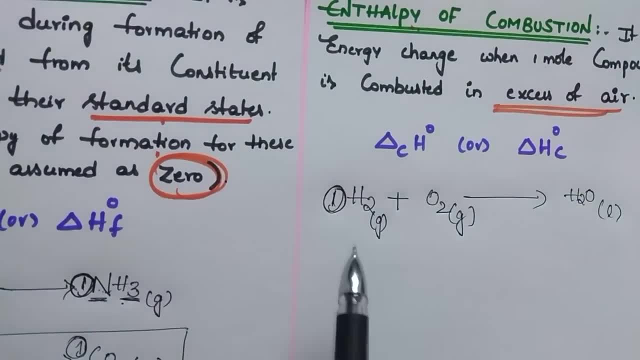 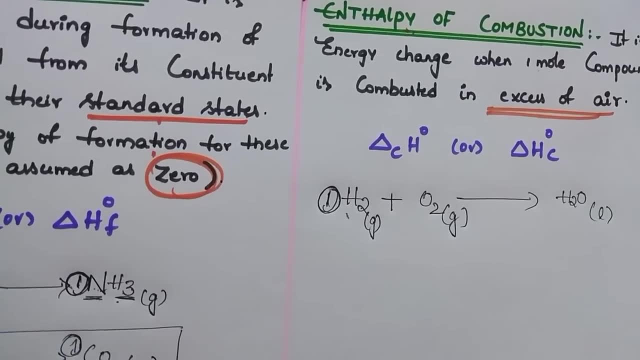 because we want to combust only 1 mole of a compound. Now, with respect to this balance, the remaining Got the clarity. students, What is the trick Here, with respect to product, Here, with respect to reactant, you have to balance the reaction. Next, how many oxygens? 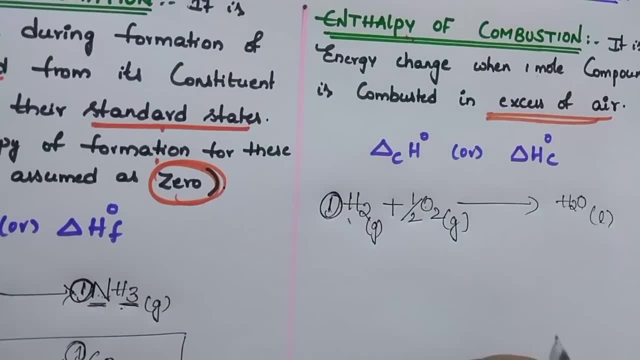 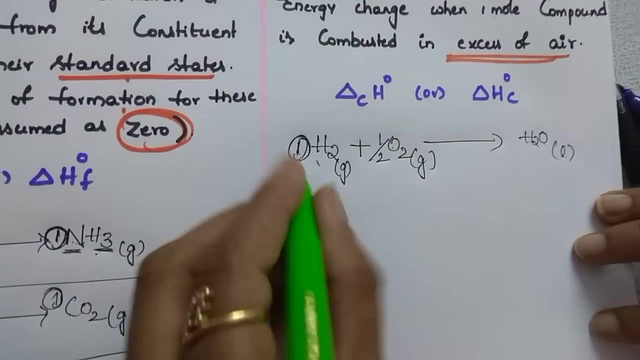 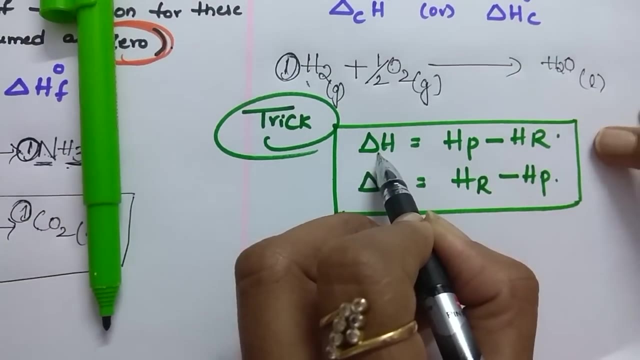 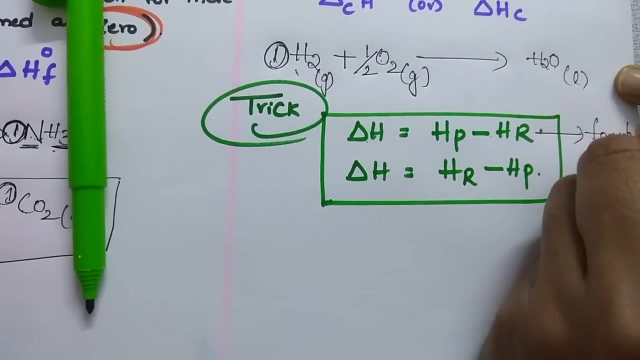 are there Only 1. Here, 2. So take half O2.. This is the standard equation. Now I am going to take the most important trick. See this: Delta H is equal to product enthalpy minus reactant enthalpy. This is, in terms of formation, Very, very important. And delta H is equal. 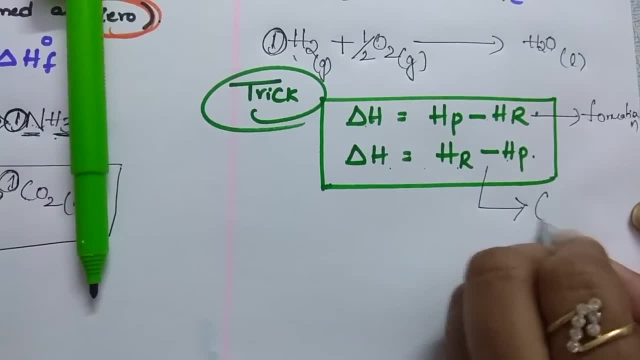 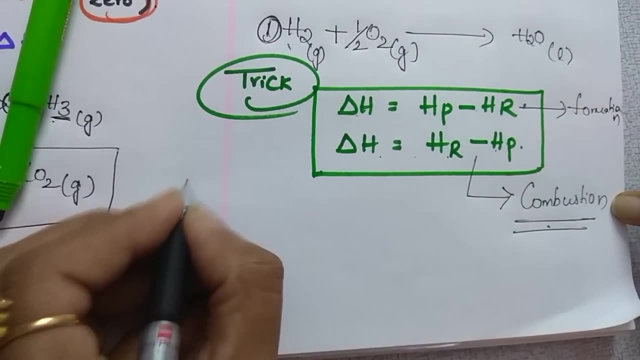 to reactant enthalpy minus product enthalpy. This is for combustion. While solving numericals, you have to keep this in mind and you have to solve it. So let's solve it, So let's solve. Suppose, see this reaction: A is converting into B, X moles of A converts into Y moles. 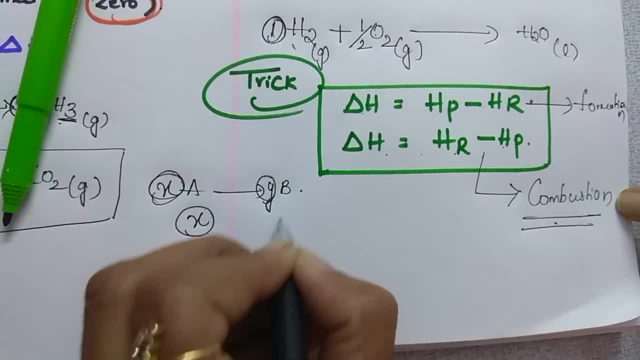 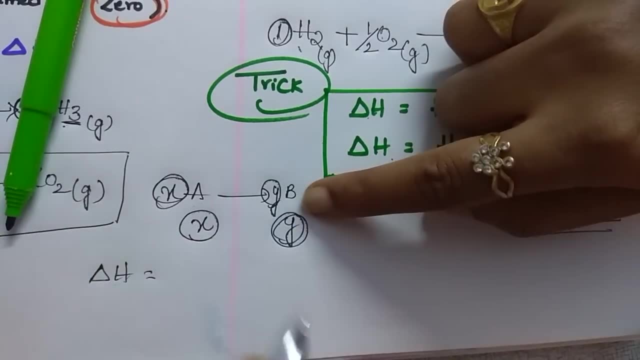 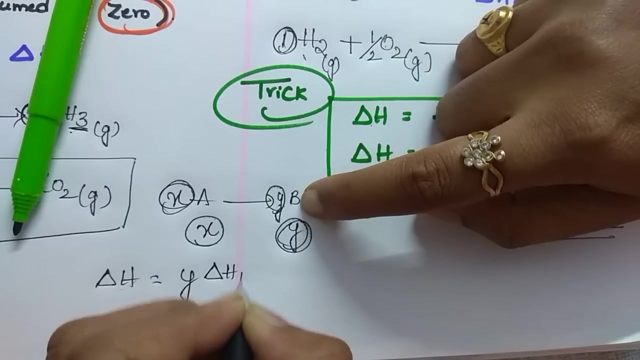 of B. What is the stoichiometric coefficient here? X. What is the stoichiometric coefficient? is Y. Now how to write the reaction for this? Delta H is equal to enthalpy of product. How many moles Y? moles of B. So I will write: delta H B minus X. moles of delta H A- Clear. 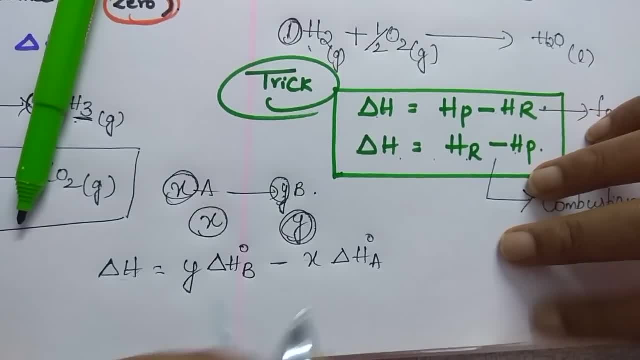 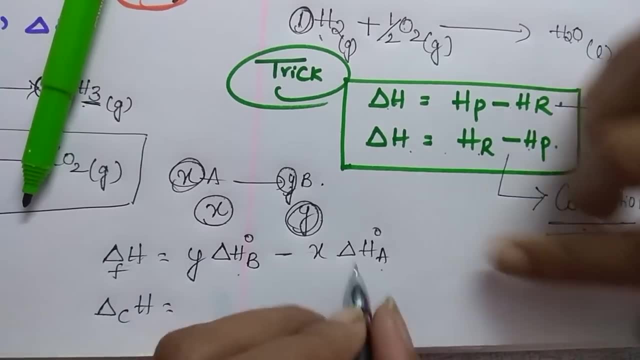 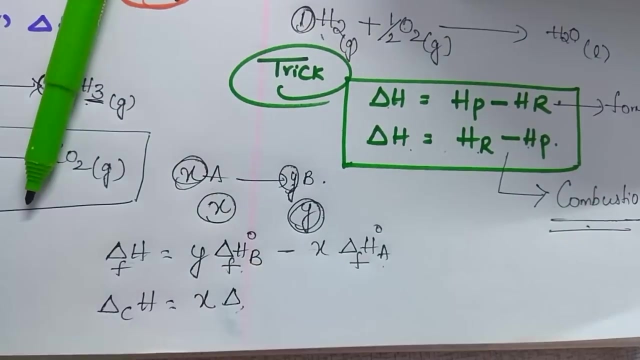 standard conditions. H naught, Here also H naught. This is for formation. Delta F of H, Now delta C of H, Combustion- How to write Products, reactants minus product X, moles of enthalpy of. This is for formation, right. So write F here. Combustion C of H. A naught. 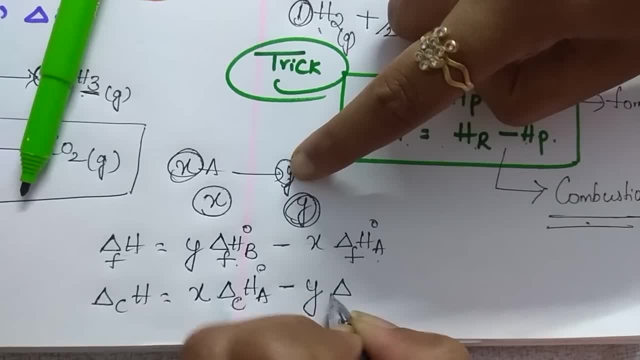 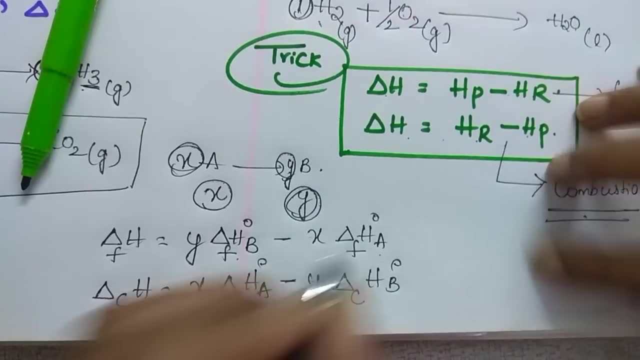 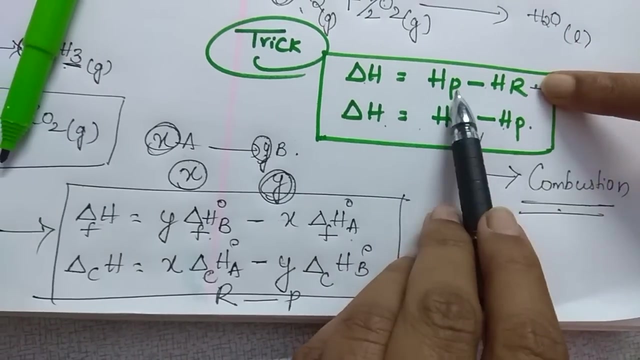 minus Y moles of delta combustion: H B naught. Y reactants minus H A- naught. So this is products. This is important. This is while doing theory questions. you have to write all this, But while doing the numericals directly, take product minus reactant for formation. 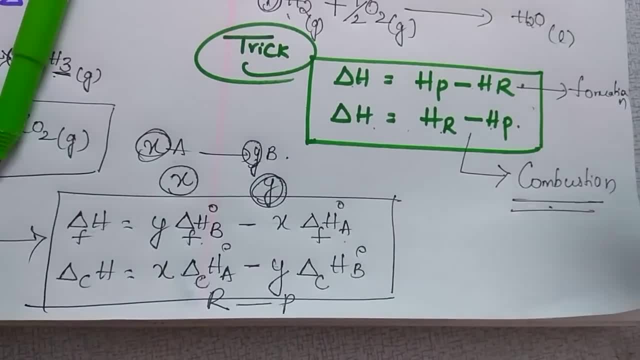 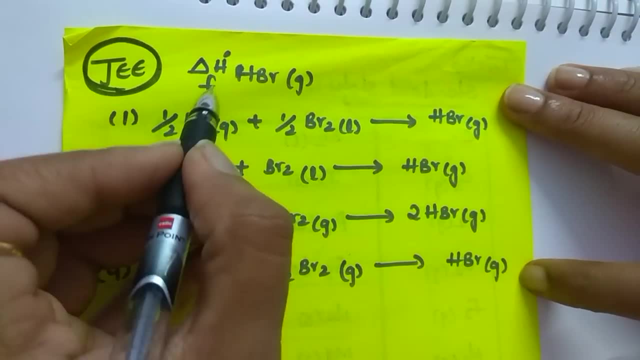 and reactant minus products for combustion. and do the numericals? Now I am going to discuss the most important numericals. Let us see one of the J equation. The question is: what is the correct expression for the formation of standard enthalpy of formation? 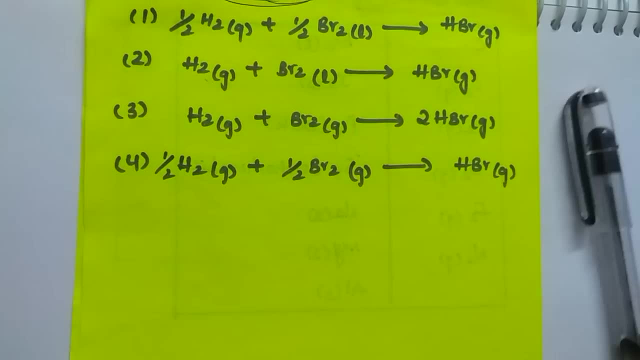 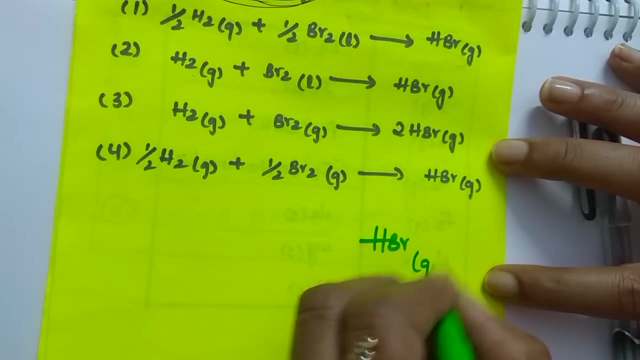 of HBR: See students HBR formation. we want. So write it in product side: HBR. in which state we want? We want in gaseous state. Take it in gaseous state. What are the elements which is having hydrogen? 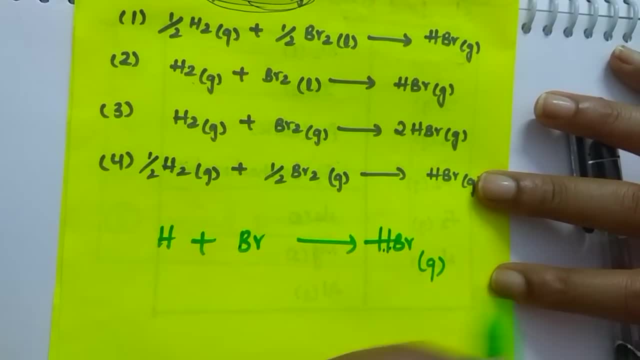 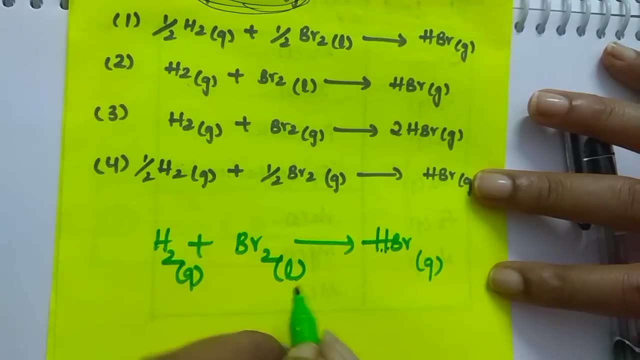 and what is the other element which is having bromine Clear And in nature, how it exists: H2 and it exists as Br2.. This is in gaseous state. This will be in liquid state. Most important, I gave you the data already And you have to balance the reaction Always. you. 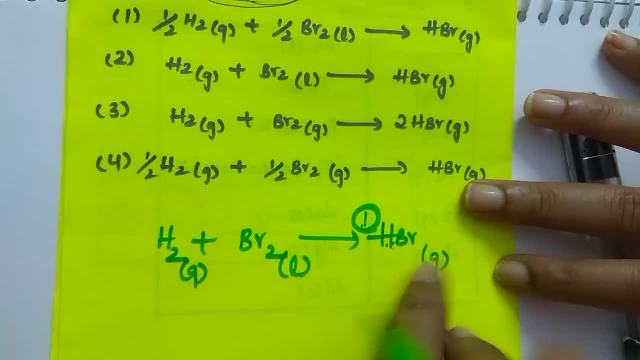 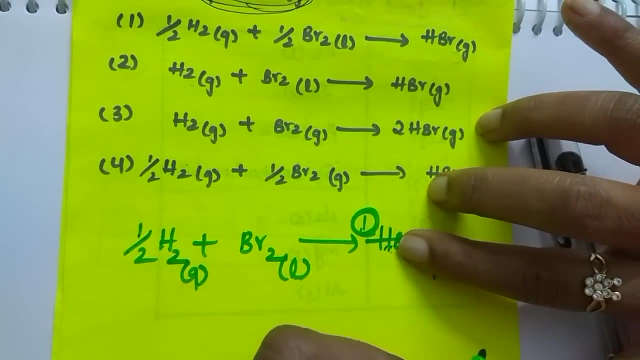 have to consider for one mole of formation, And if you take two mole, that is not standard enthalpy of formation. Only for one mole, Then how many hydrogens we want? Only one, So take it as half. And only one Br, So take. 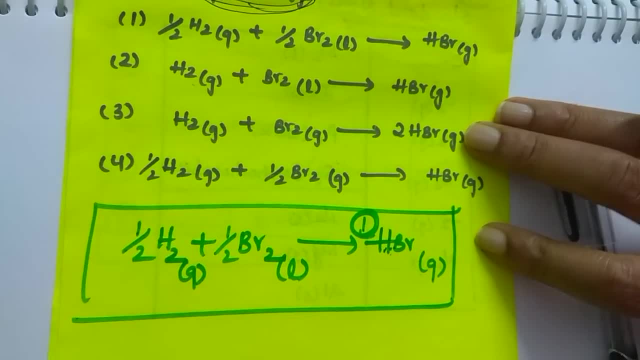 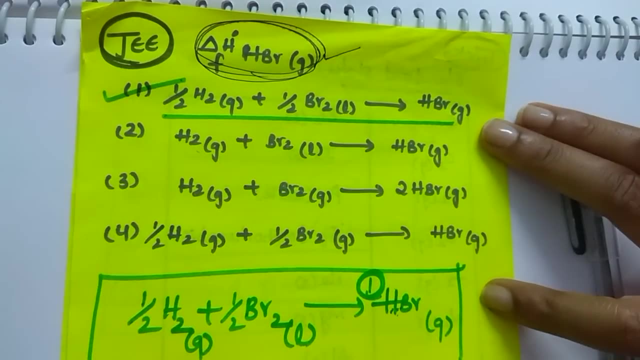 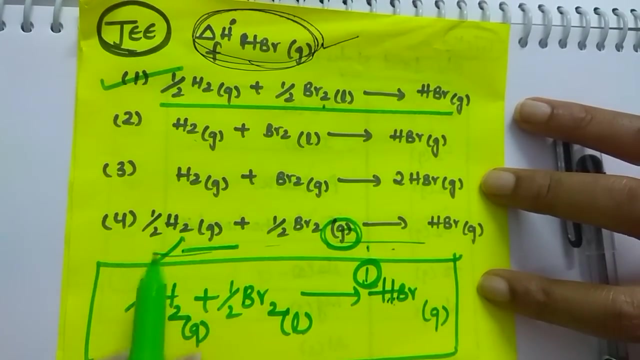 it as half. That's it. You solve this J equation very easily. What is the correct option for this? This is the correct option. If you mark this, both look same. But here bromine is in liquid state, Here it is in gaseous state. If you mark this, this is the wrong Clear. 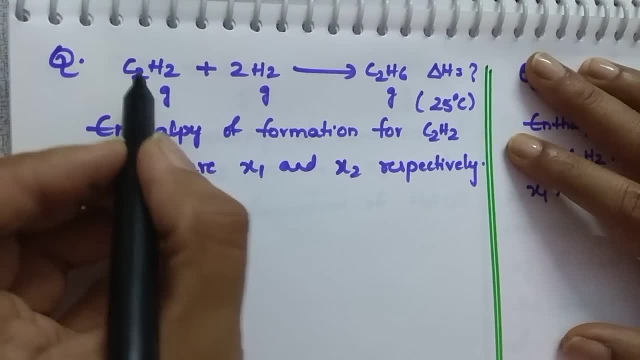 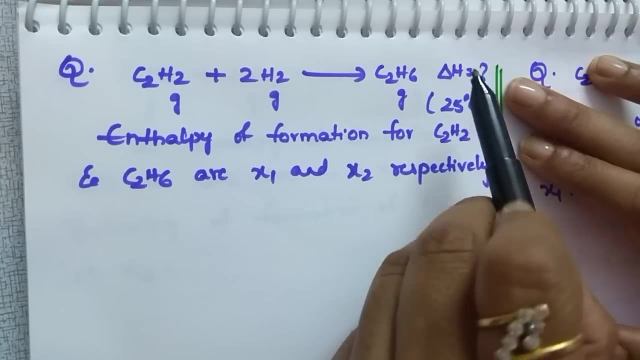 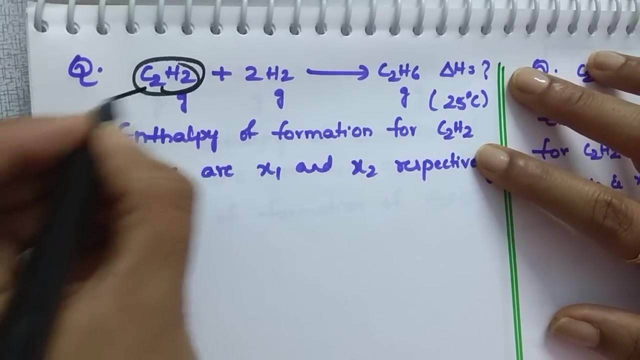 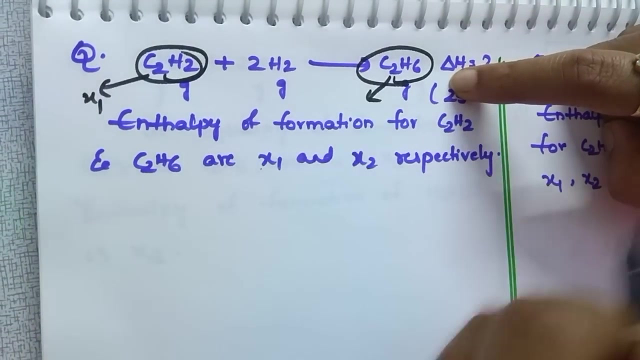 Believe me, See this question, students. We are going to calculate this reaction. Enthalpy of formation of this is given as X1 and enthalpy of formation of C2H6 is given as X2.. What you have to do is first write the reaction. Which reaction? this? 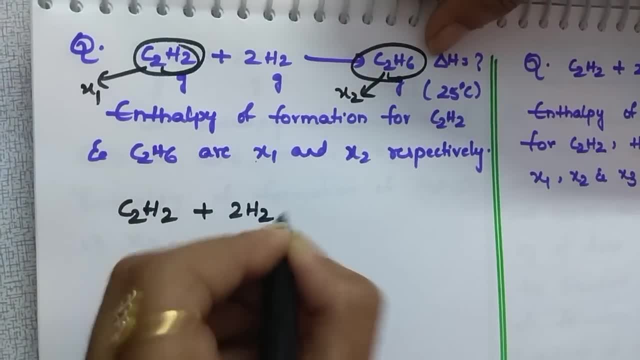 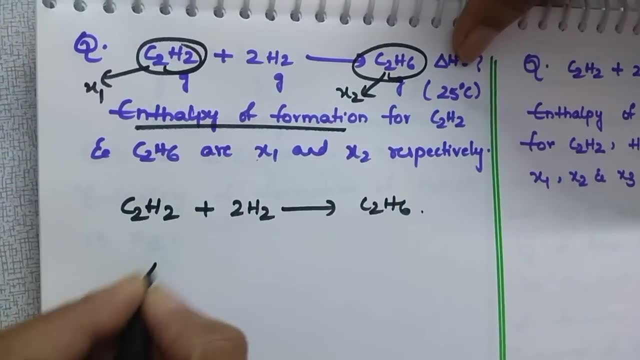 reaction, C2H2 plus 2H2 gives rise to C2H6.. What I taught you: if it is enthalpy of formation, you have to write the formula, as delta H is equal to enthalpy of products minus enthalpy of. 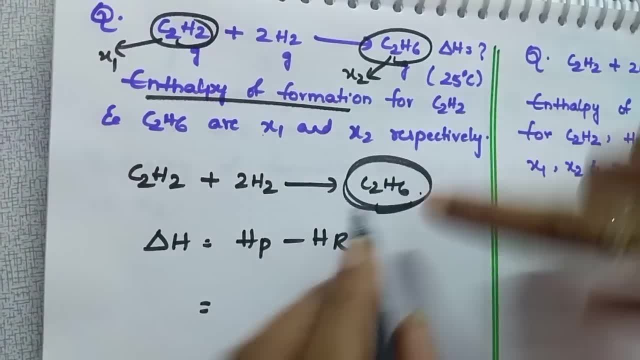 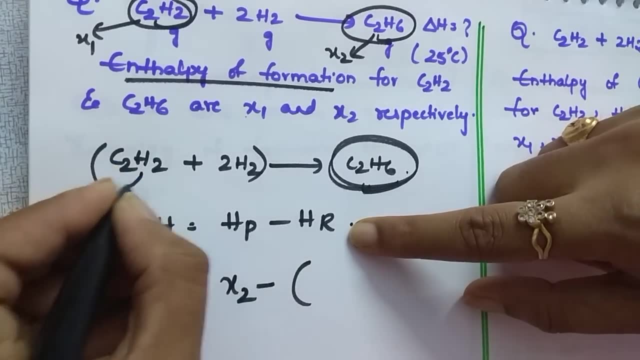 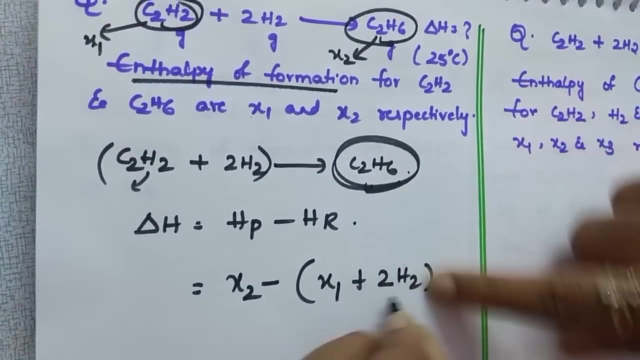 reactants. Short way is product is how much enthalpy of product is X2 minus reactants? is these two Means, suppose, if you consider this, how much is given X1 plus 2 into enthalpy of hydrogen? but here enthalpy of hydrogen is not. I am not writing in expression form because it is waste. 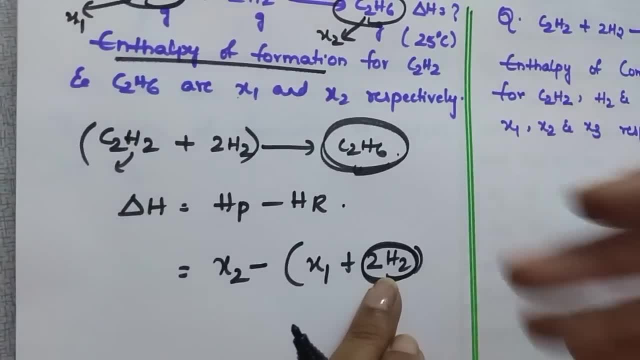 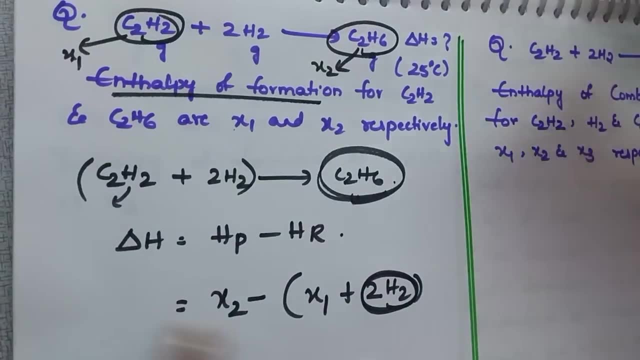 of your time in objective examination. If you want to do for theory exams, then go through the formula which I gave here. Understand: in this formula you write So 2 into H2 and H2 hydrogen is not given in question. What you have to do 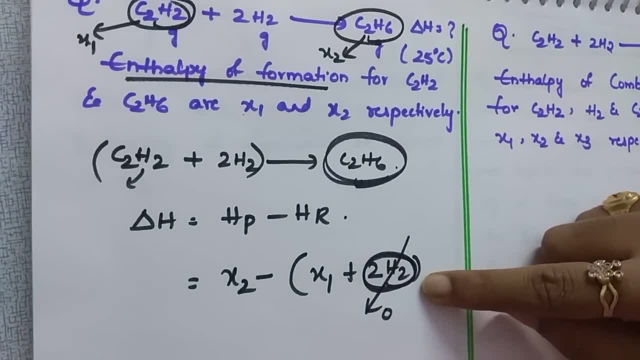 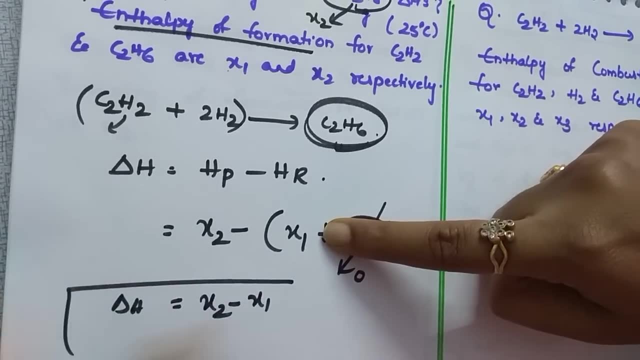 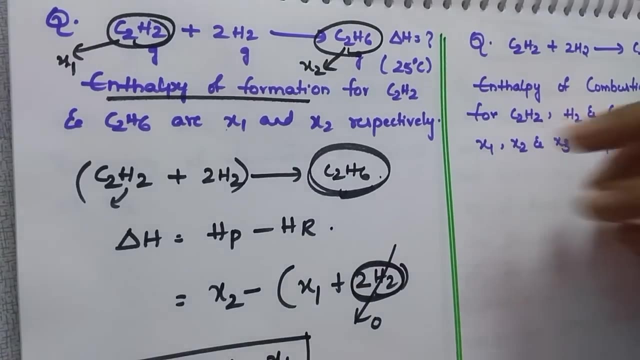 Is hydrogen present in their standard states, then it is assumed as zero. What is the formula, students? then X2 minus X1. Here I didn't take the values, just I am taking as X2 and X1. to make you clear of this concept, In next video I will take the best examples and I will do the 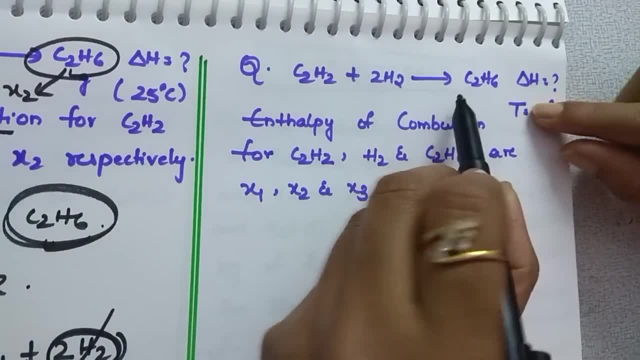 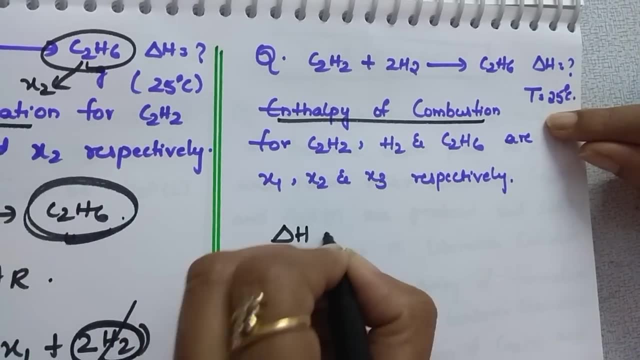 problems. Coming to the next one, To the same reaction, you have to find delta H, but enthalpy of combustion is asking. Then, what is the formula? enthalpy of combustion You have to do. reactants minus products is the formula. This is important. What is enthalpy? 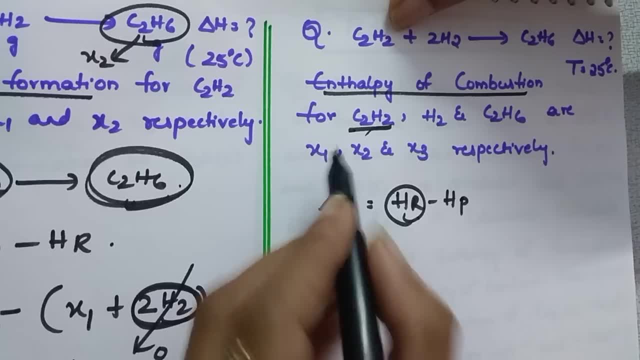 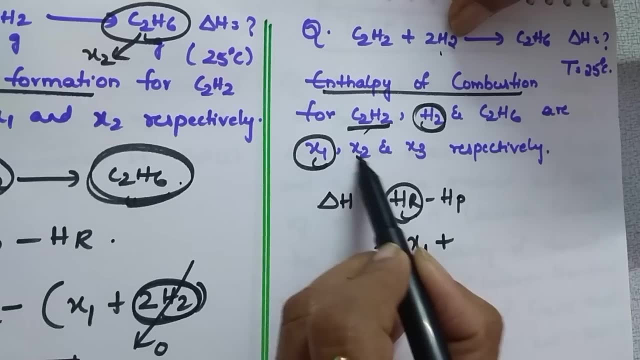 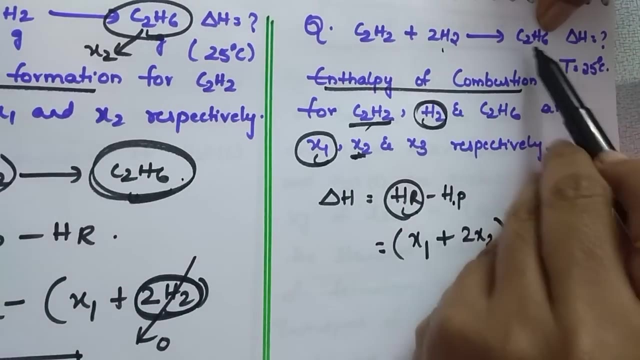 of reactants. C2H2 is given as how much X1 plus 2 into hydrogen is considered as X2.. So 2 into X2. this is reactants minus products. What is the enthalpy of combustion of C2H6?? 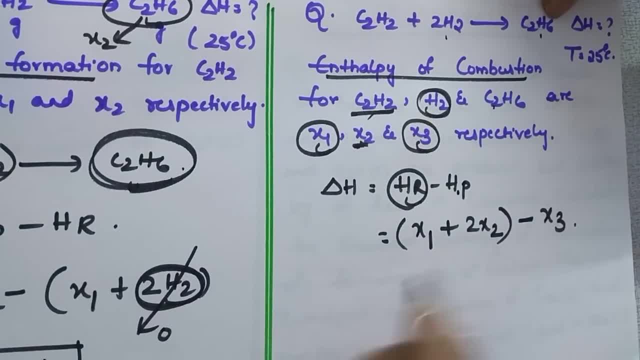 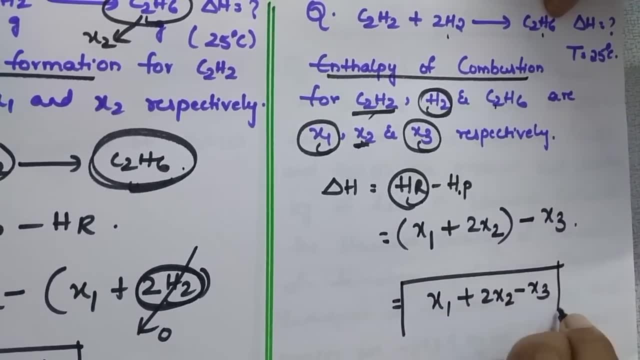 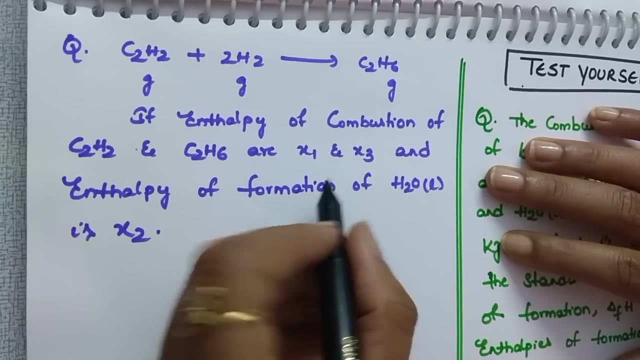 C2H6 is given as X3.. What is the formula? X1 plus 2 into X2 minus X3 is your formula? See this question, Same question, but the data is different In this question. enthalpy of combustion of this is. 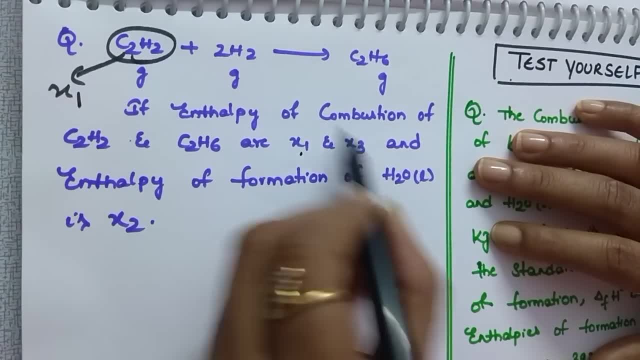 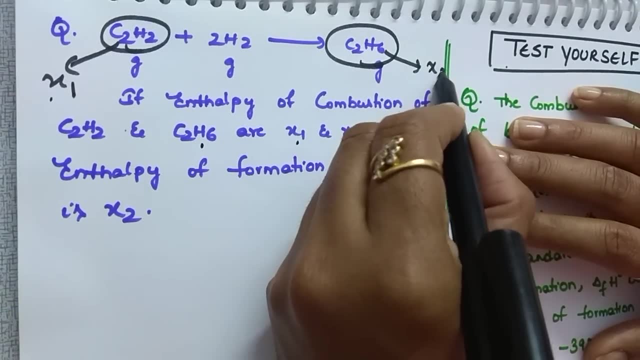 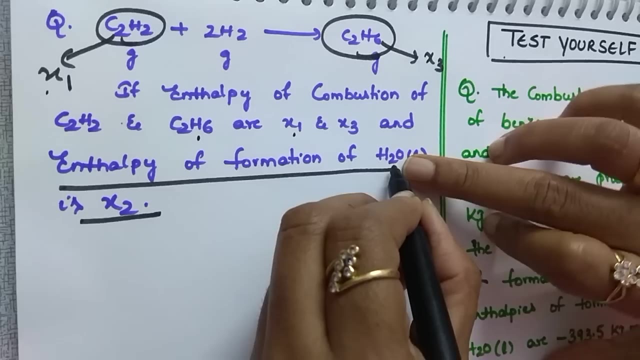 given as C2H2 is given as X1 and enthalpy of combustion of C2H6, H2 is given as X1 and C2H6 is given as X3. What you have to do? Enthalpy of formation of H2O is given, So write the expression. 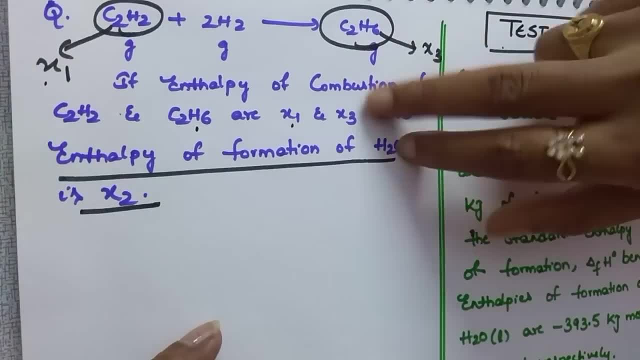 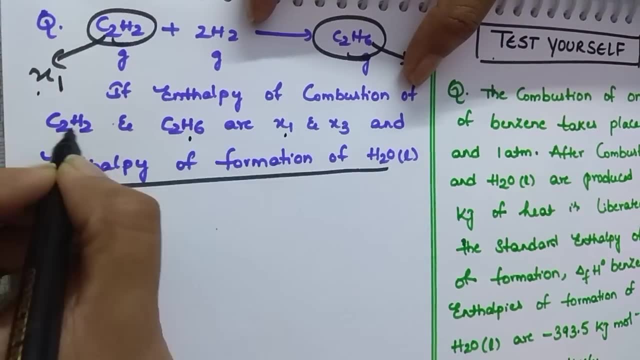 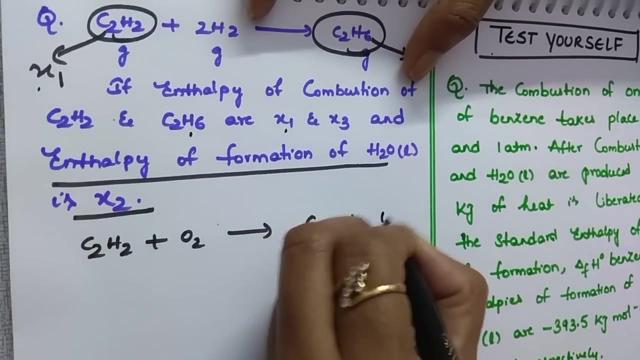 Every data you can write as an expression Directly. also you can substitute, but here, in order to make you clear, I am writing in the form of expression: Enthalpy of combustion of C2H2.. What it means: C2H2 plus O2 gives rise to CO2 plus H2O because we do combustion. 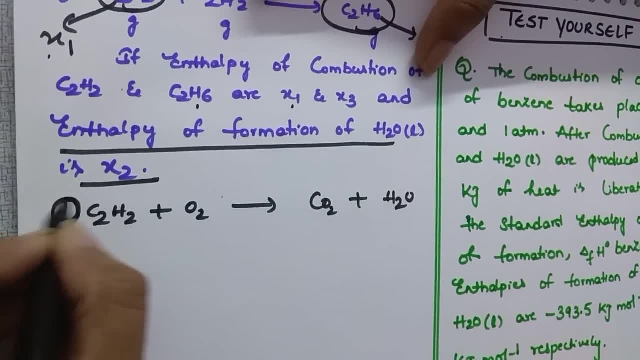 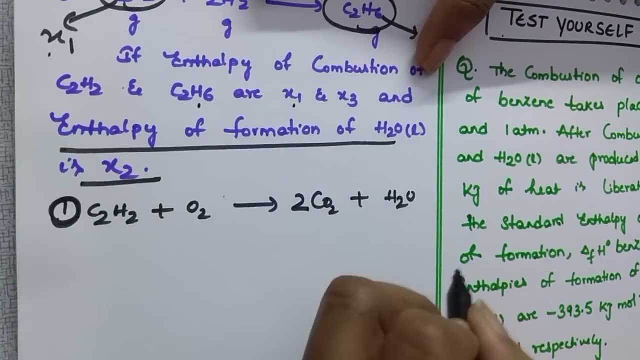 in the presence of oxygen. All we do this. So 1 mole of this means balance with respect to C2H2.. How many carbons? 2 carbons. How many hydrogens? 2 hydrogens Balanced. How many oxygens? 2 2s are 4 and. 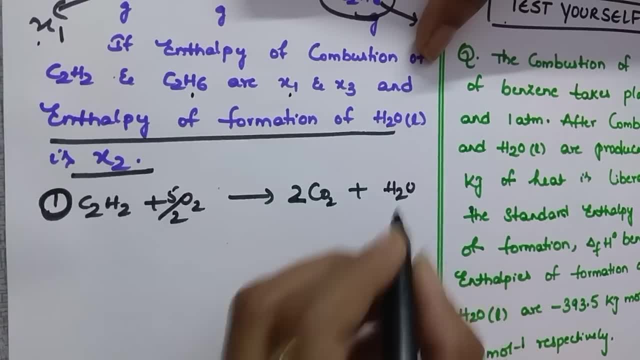 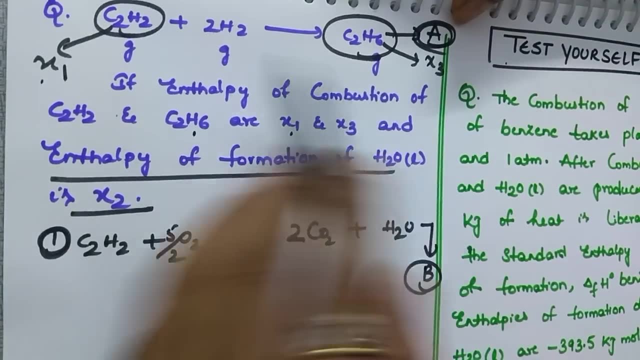 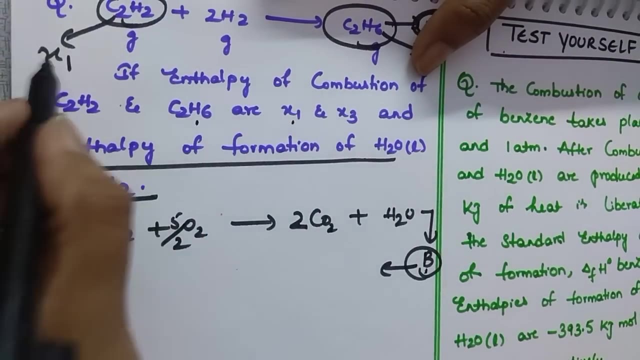 1, 5.. So 5 by 2.. This is a balanced equation. Name this expression as, suppose B. Consider this as A reaction. We want to find delta H of combustion to this reaction. So I am considering it as a, B, and what is the combustion value given for this? as X1. 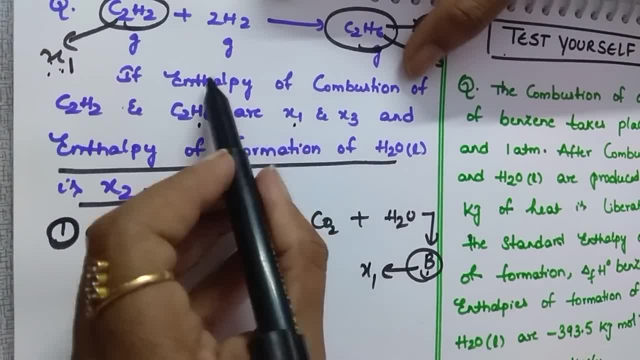 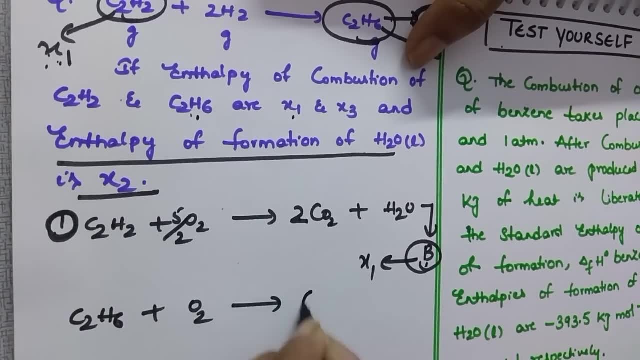 This is given in the question as X1.. Next one: Enthalpy of combustion of C2H6.. Write this: C2H6 plus O2 gives rise to CO2 plus H2O. Students, to make you clear, I am balancing. 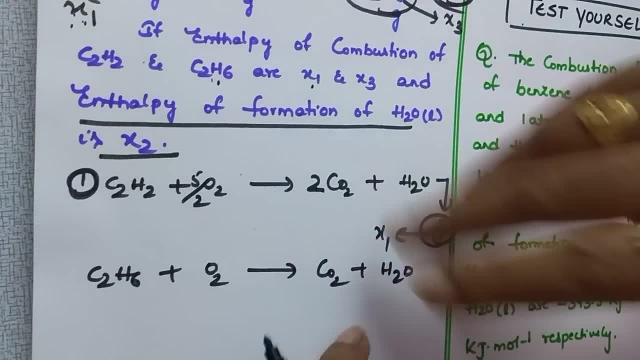 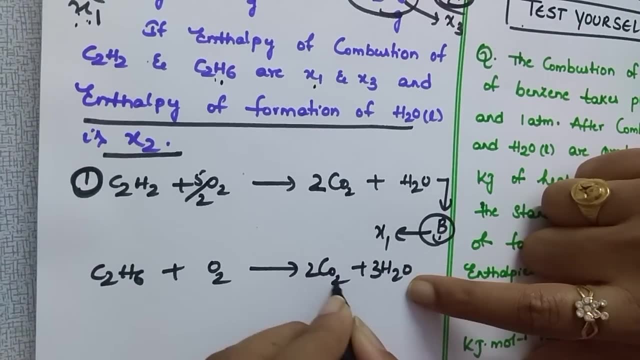 but in short, without balancing this and all you can do directly: How many carbons? 2 carbons- and how many hydrogens? 6. so 3 and 2, 2s are 4, 7, 7 by 2. This is the equation Name. it. 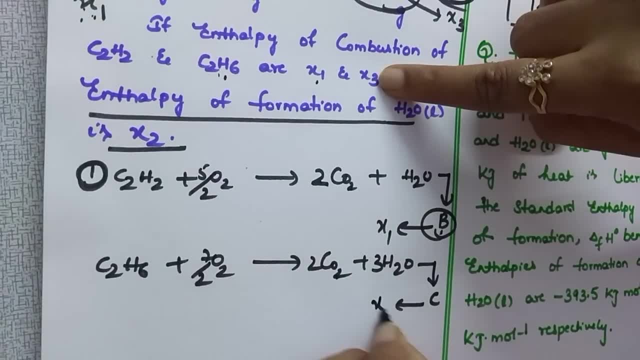 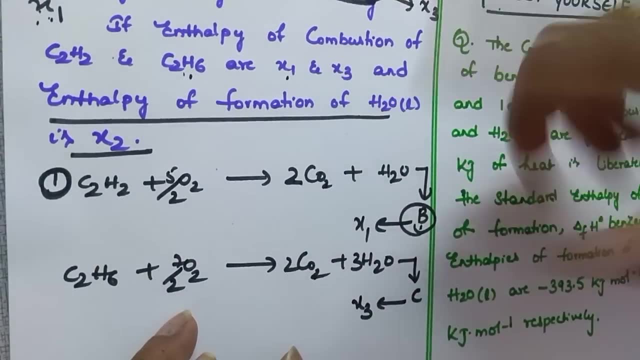 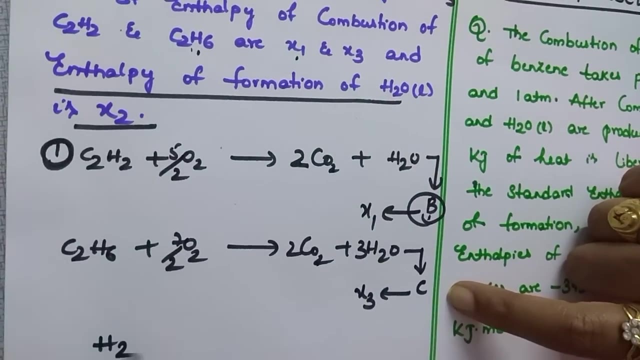 as C, Assuming this enthalpy of combustion considered as X3.. This is easy. Directly you can substitute Why I am discussing because of this enthalpy of formation is given 2 in terms of combustion, 1 in terms of formation. How to do is write the formation: H2 plus half O2 gives rise to 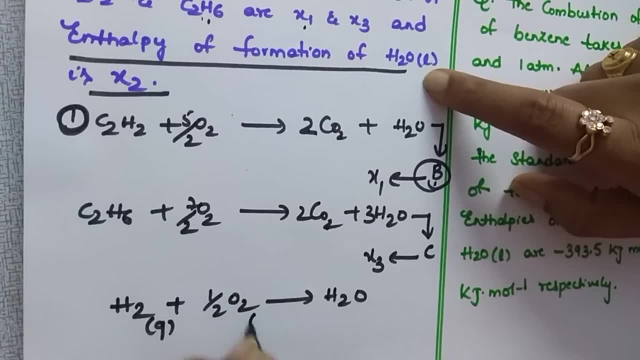 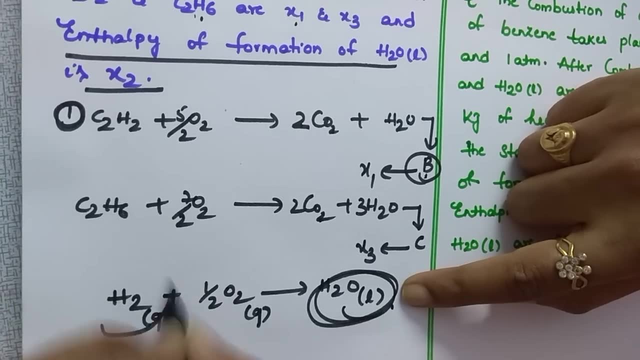 H2O. Now this is in gaseous Write, its expression given in liquid state Here. observe here: enthalpy of formation of H2O is nothing but enthalpy of formation of H2O is nothing but enthalpy of combustion of H2.. That's it. Both are same. Then in this question you can directly. 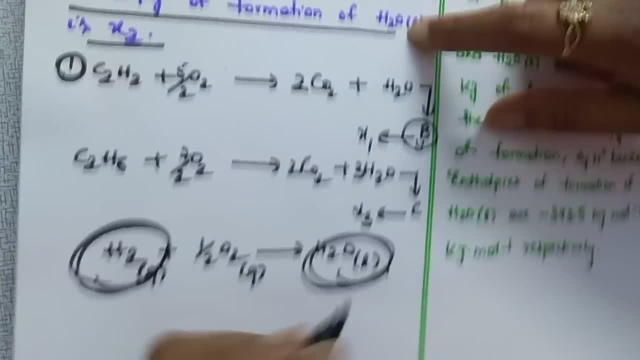 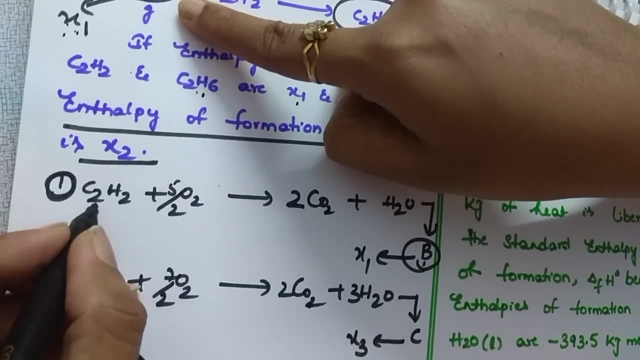 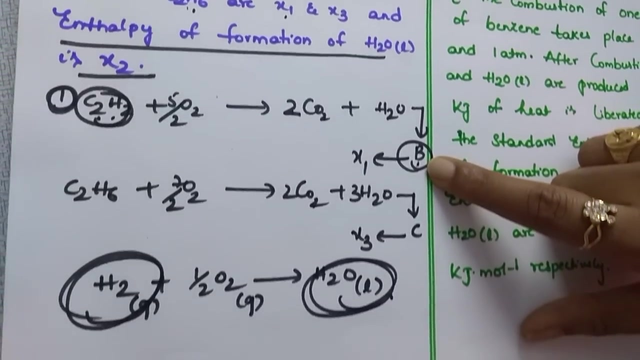 substitute the value of X2.. Now write down: delta: H is equal to. We want C2H2 in reactant set. So here in expression B it is there in reactant set. 1 mole, Here also 1 mole. So take it as B into 1, plus here H2.. So how many are there? 2 hydrogens is there in reactant. 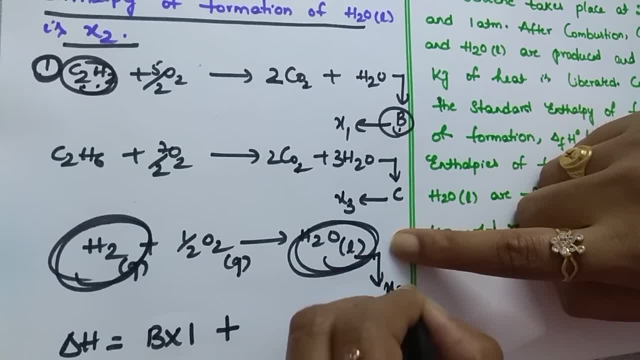 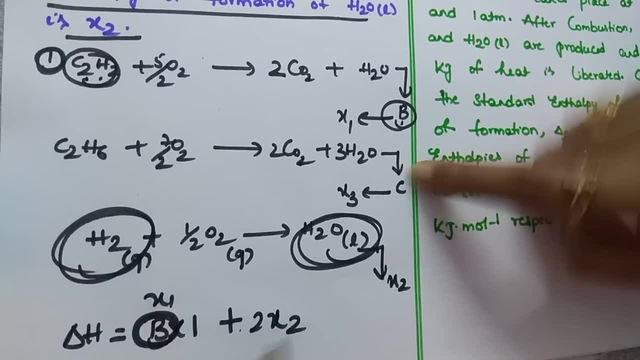 set Here only 1 hydrogen. So take this expression 2 times 2 into X2.. B is how much Students X1. So X1 plus 2 into X2.. Here C2H6 is given in reactant set, Product set. Here it is in.